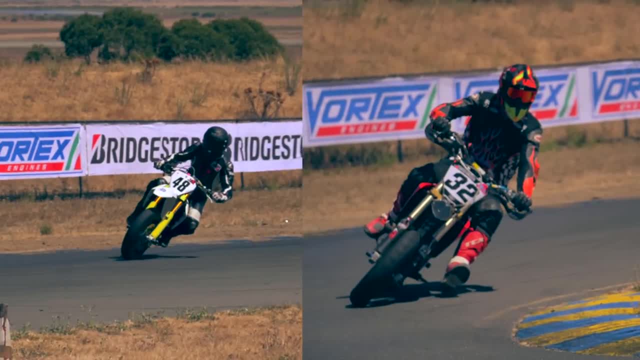 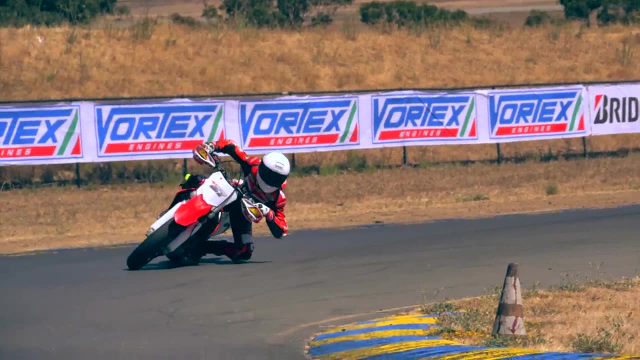 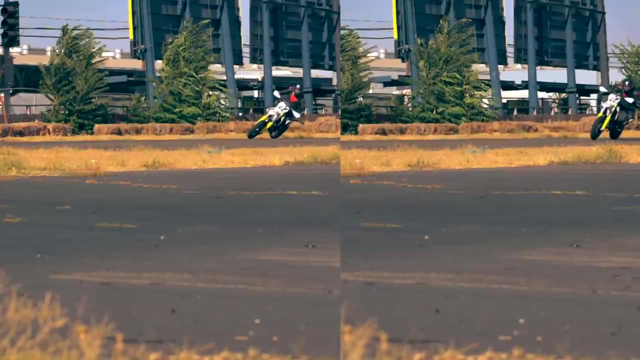 various styles. This is especially true in Supermoto. There you will see some riders pushing the bike down with their foot out while others are hanging off. Then there are those like me who mix all the styles. I'm pretty sure a beginner watching me riding on a supermoto track would be. 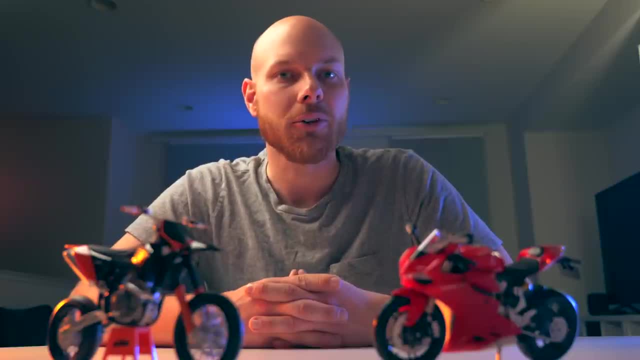 very confused. In order for you to understand the answers that I'm going to give to the questions that I post in the beginning of the video, it's important that you understand some basic concepts of cornering technique and chassis geometry. Therefore, I'm going to walk through. 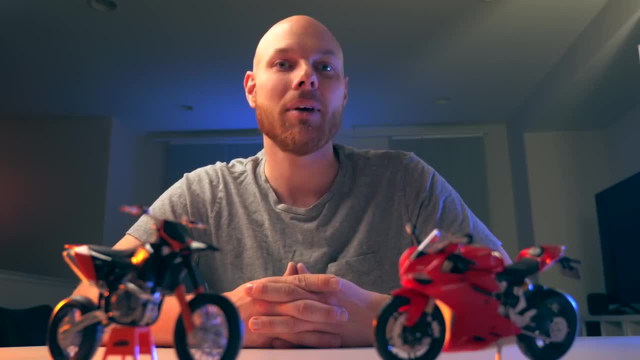 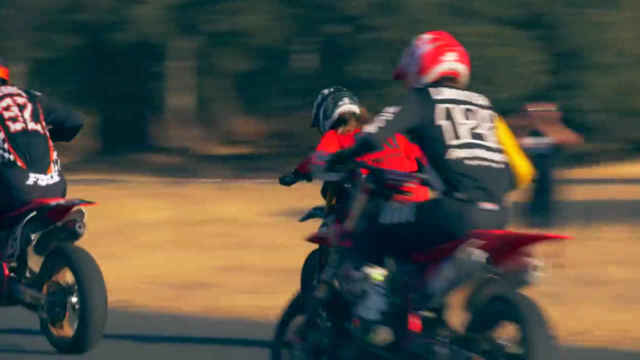 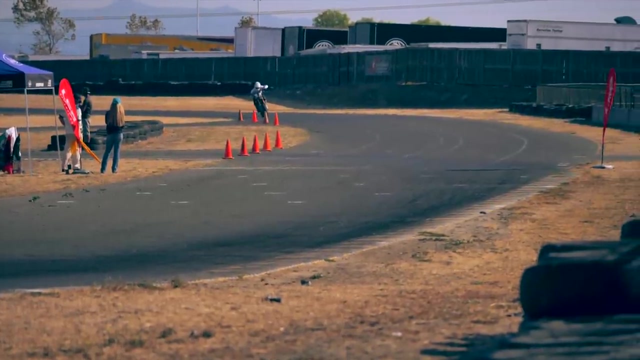 a corner, step by step, explaining each step in detail. These steps apply to superbike racing, MotoGP and the asphalt sections of Supermoto. To keep things simple, the corner we're going to look at is going to be at the end of a straight. This is an important assumption, because it 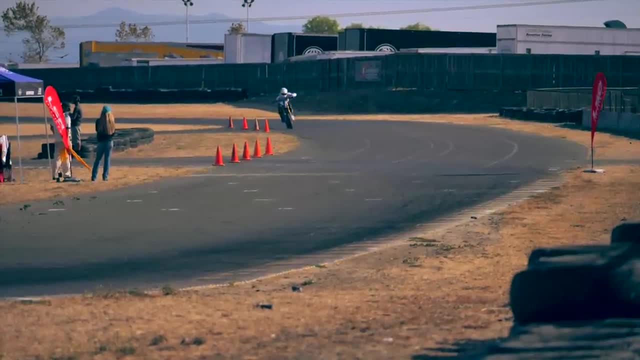 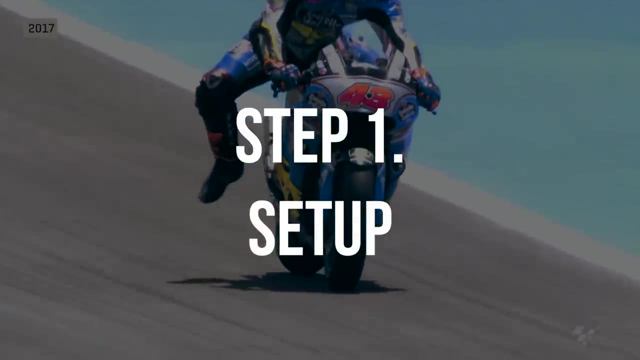 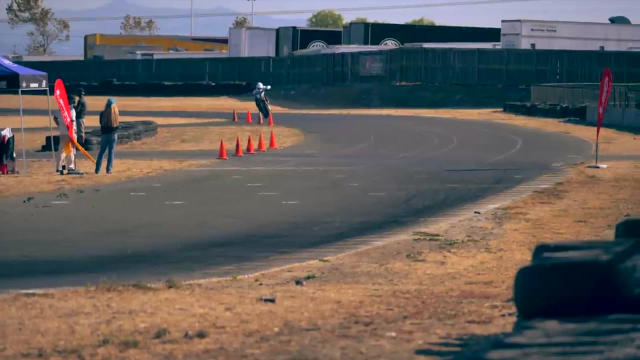 affects what body position the rider has and what state the bike's chassis is in. when moving the bike, The rider is accelerating on the other side, towards the corner. Step 1 is setup Before entering the brake zone. the rider has a tucked body position to minimize aerodynamic drag. 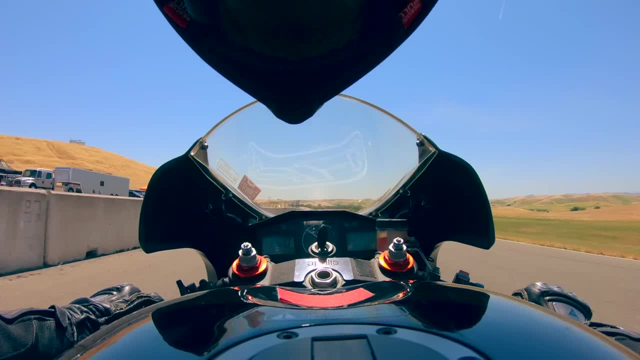 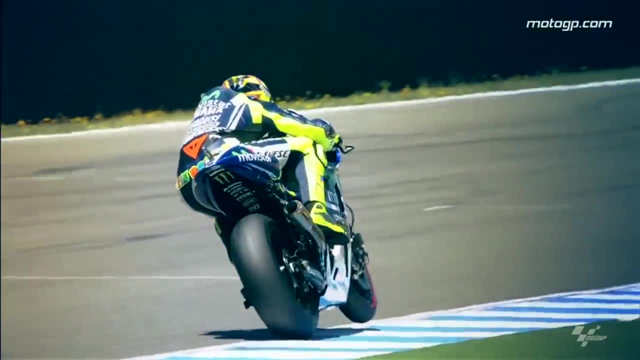 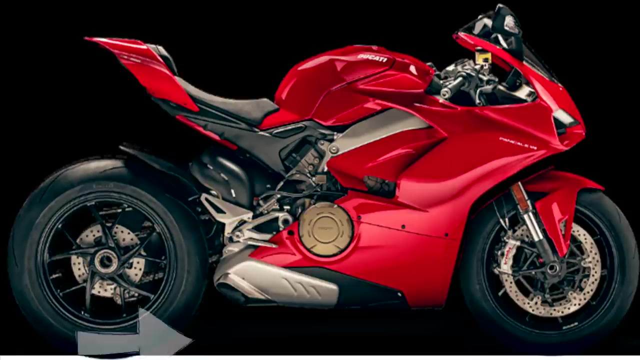 and maximize their top speed. The rider is accelerating hard, which extends both the front and rear suspension. The front extends because of load transfer, The rear extends because of chassis geometry, So the swingarm has an angle which you could say rear wheel, under the bike when you accelerate. Furthermore, the chain pulls on the axle at an 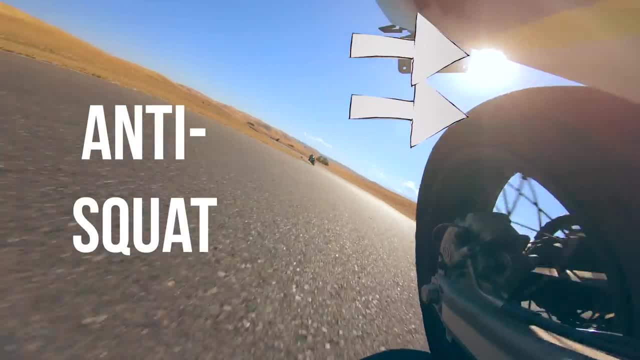 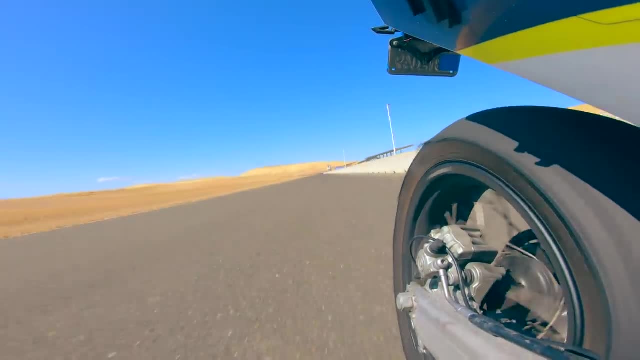 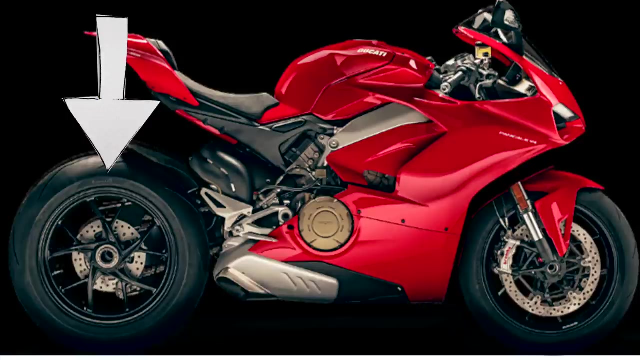 angle which adds on to this force. This is called anti-squat, and the chassis is designed that way so that the rear suspension does not run out of travel when accelerating Because of the way that the swing arm pivots. extending the rear suspension will decrease the total wheelbase of the motorcycle. 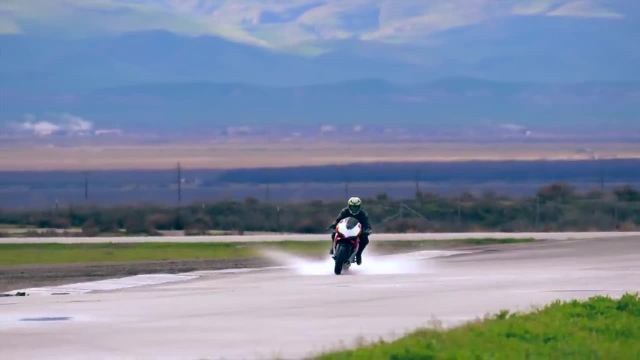 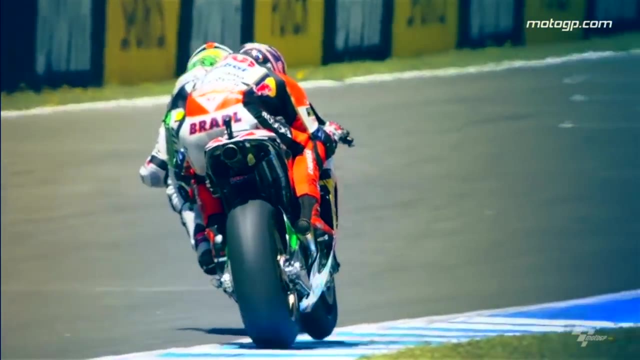 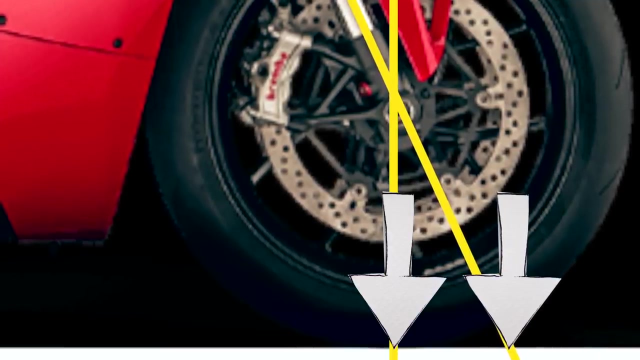 This will decrease the stability of the motorcycle, which is not necessarily something desirable, but a trade-off one might be willing to take in order to get the anti-squat characteristic using simple geometry. When the front fork extends, this increases the trail of the motorcycle, which 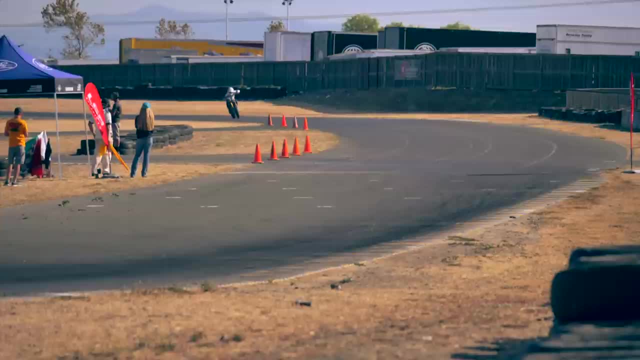 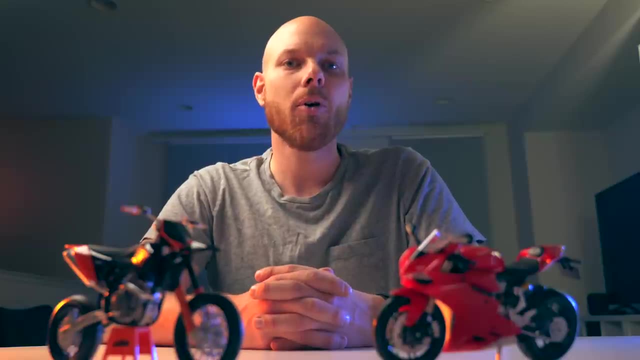 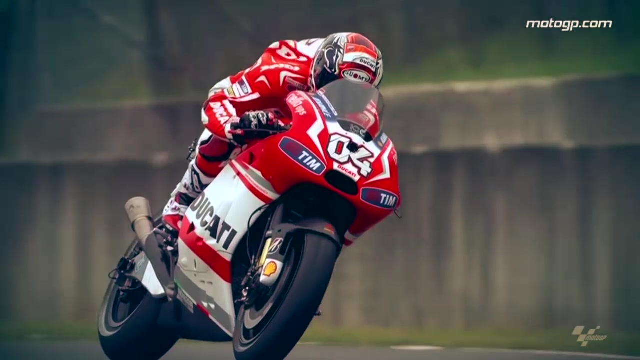 increases the overall stability of the motorcycle. In this state, the motorcycle is very stable, but also requires more force to steer. If you want a more in-depth explanation of motorcycle geometry, check out the video that I did on the subject right here. Okay, so the rider is tucked. 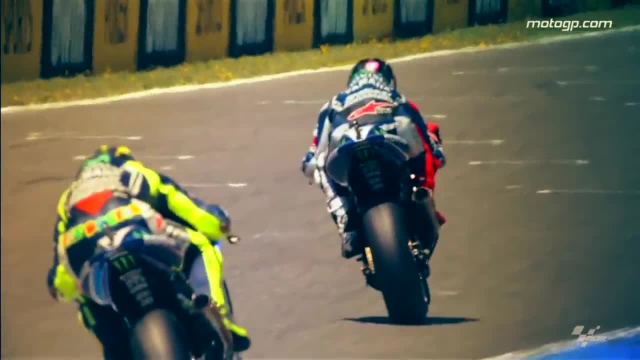 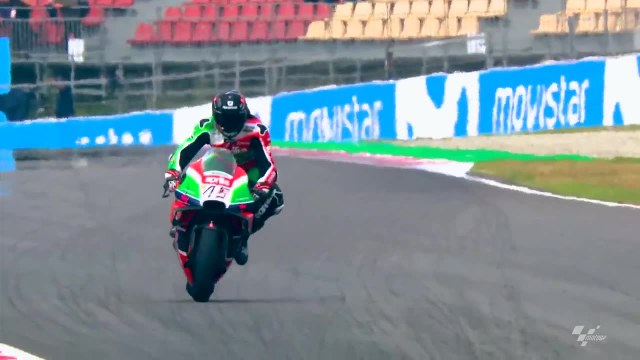 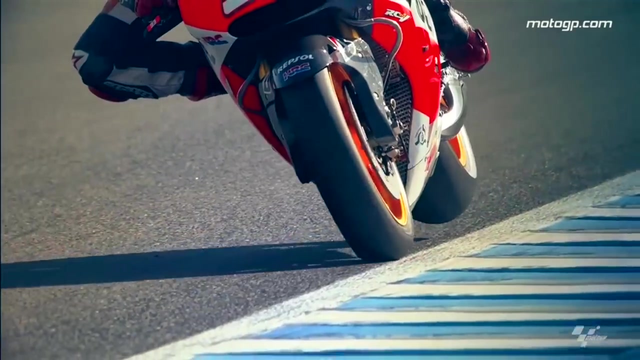 on the bike accelerating hard. The bike is as stable as it can ever be. Before or at the very beginning of entering the brake zone, the rider will set up for the corner. What this means is that they are positioning their lower and upper body for entering the corner. The reason, the 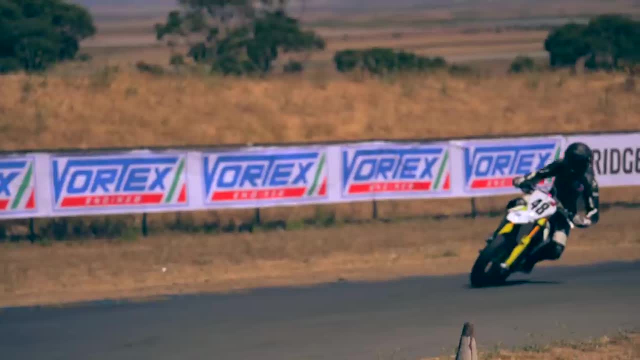 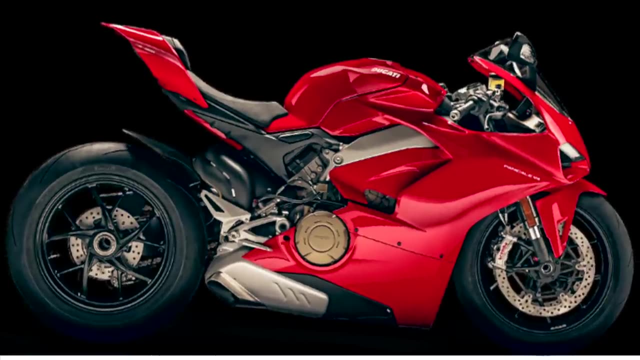 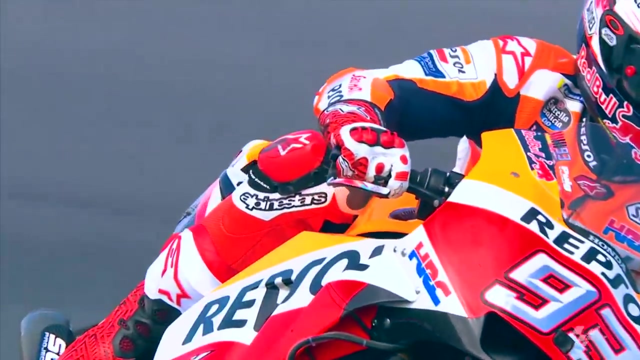 rider is setting themselves up before the corner is to keep the bike as stable as possible. As soon as the front brakes are engaged, the load will transfer forward, which will compress the front forks, decreasing the trail. This makes the bike unstable but easy to steer. Some riders use 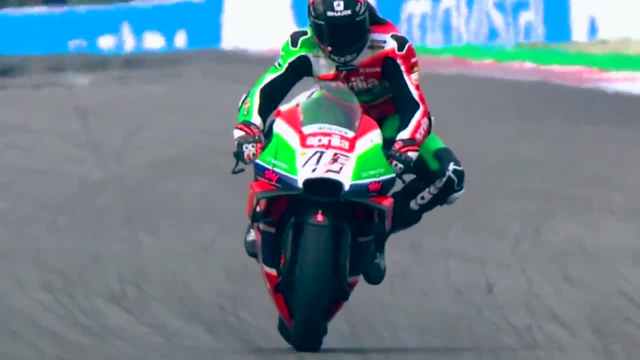 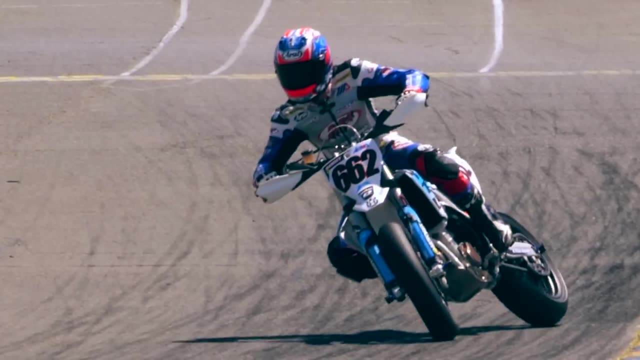 the g-forces from the initial brake input to move their lower body without much effort. Moving just when initiating the brakes will indeed make the bike slightly unstable, but also minimizes the effort needed to move. As usual in racing, it's all just a trade-off. 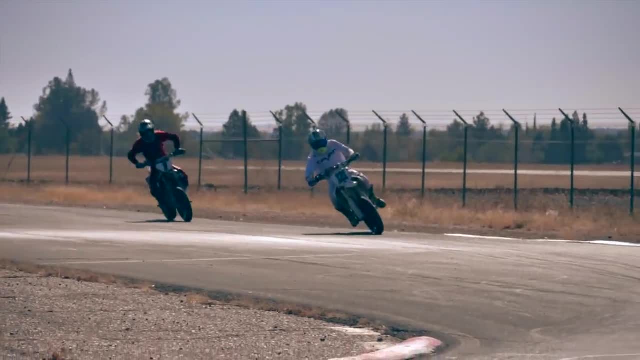 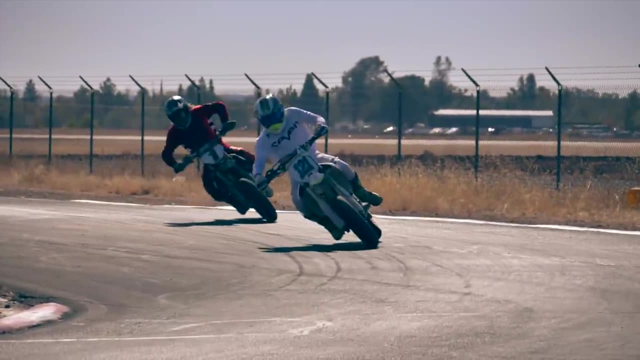 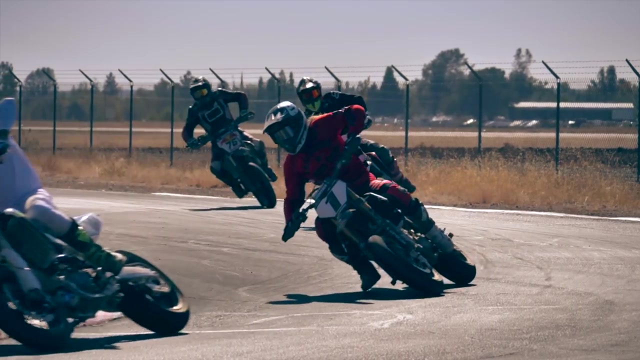 A supermotor rider that pushes the bike down beneath them, sometimes called dirt bike style cornering will move their butt out and far forward on the bike. This puts them on top of the bike, which makes it easier to control and save slides. You'll see some riders sitting all 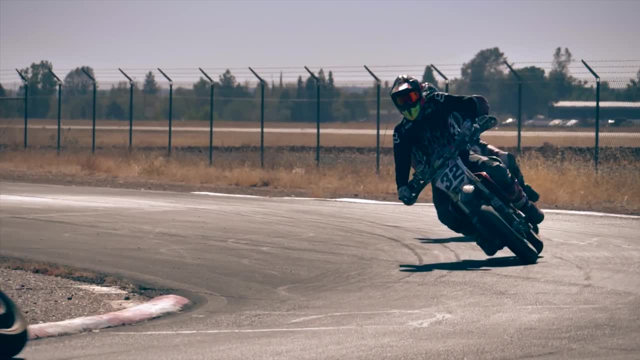 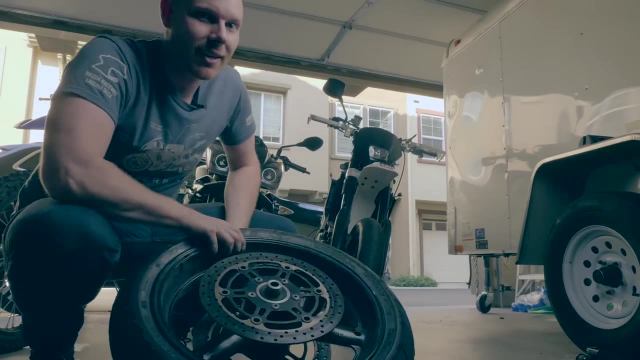 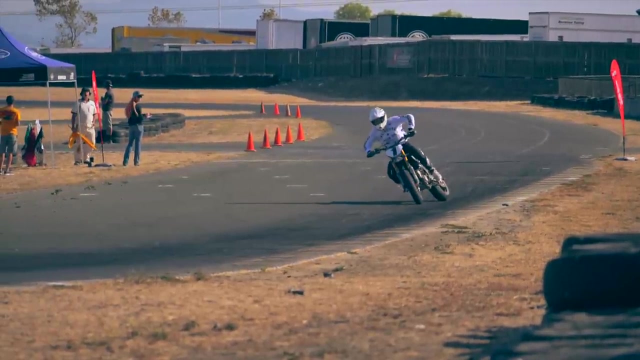 the way up on the tank. This way, they transfer load to the front tire, which will provide more traction up front and less in the rear. If you want a more in-depth explanation of tire traction, check out my video on the topic here. When the rear end is sliding, the front wheel is going to 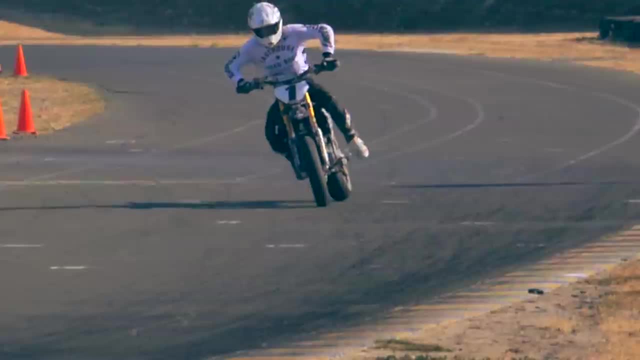 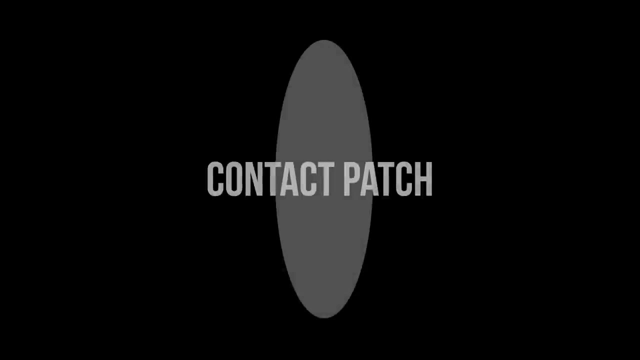 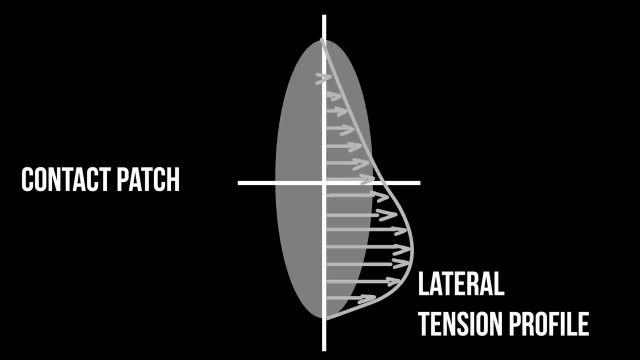 naturally counter-steer, even without rider input. This is because of the trail on the front fork and something called self-aligning torque of the front tire. The self-aligning torque is created by the pneumatic trail, which is caused by progressive build up of lateral force. 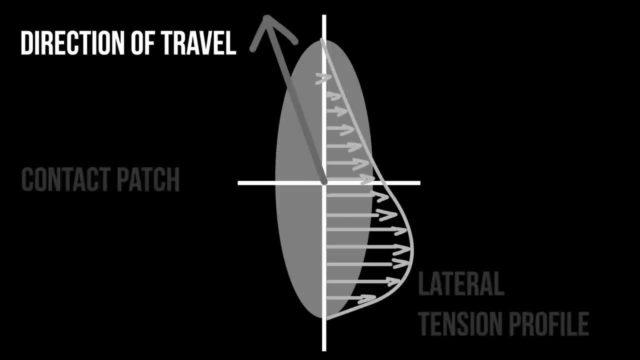 along the length of the contact patch such that lateral forces are greater towards the rear to the rear band of the front tire. If the rear end is sliding, it will turn the bike diagnosis to the CBN and turn it into a BGM. If the front wheel is healed out when the front wheel starts to start. 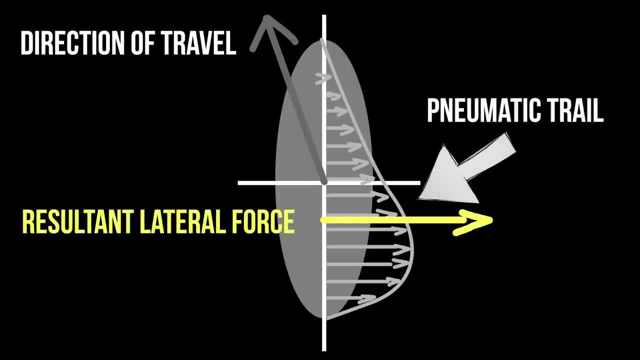 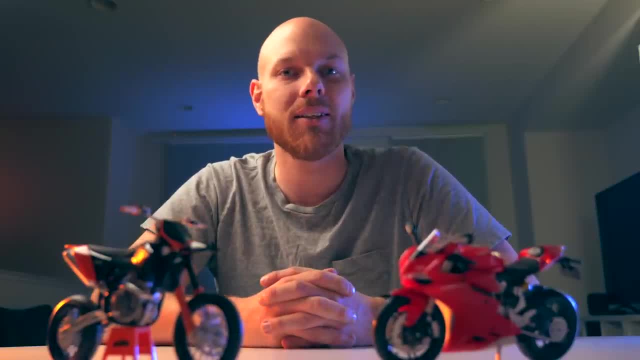 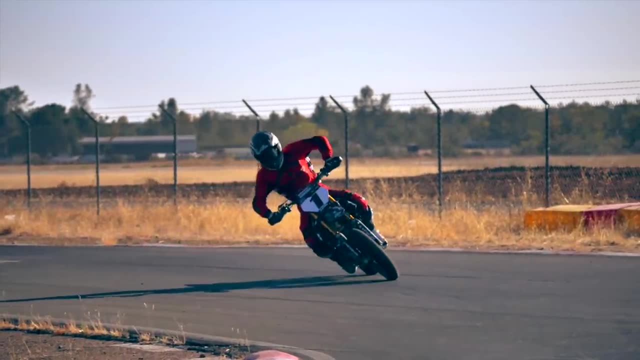 2 of the contact patch. Don't worry if you don't understand what the pneumatic trail is. I scratched my head for a long time trying to understand that subject. What you need to understand is that, in order to have maximum control over the front wheel, it is easier to sit on top of the bike. 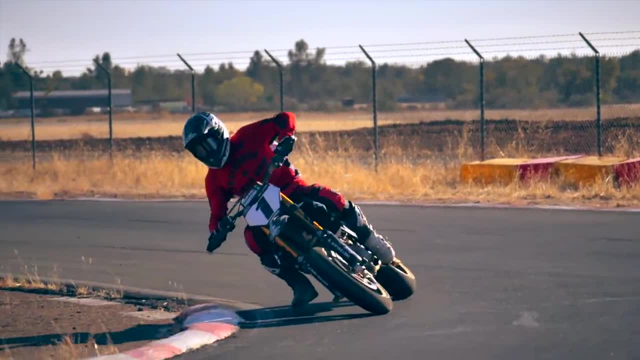 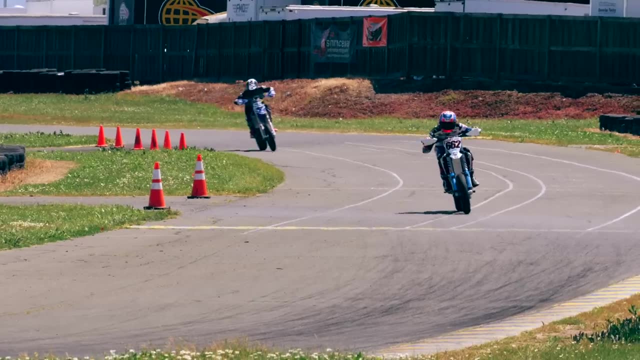 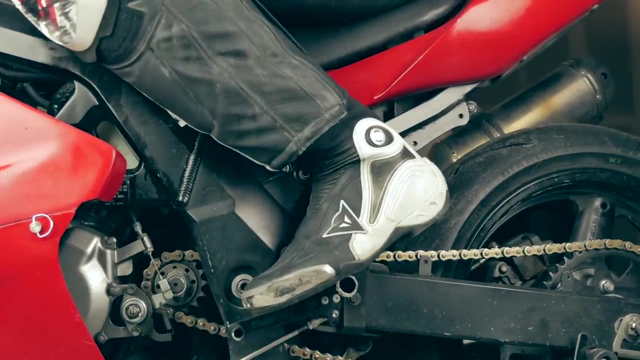 with elbows up in the air as opposed to hanging off to the inside of the bike. Step 2. Initiate braking and shift down. As soon as the rider releases the throttle, they begin braking. pull the clutch and shift down to the appropriate gear for the corner, When and how the clutch is. 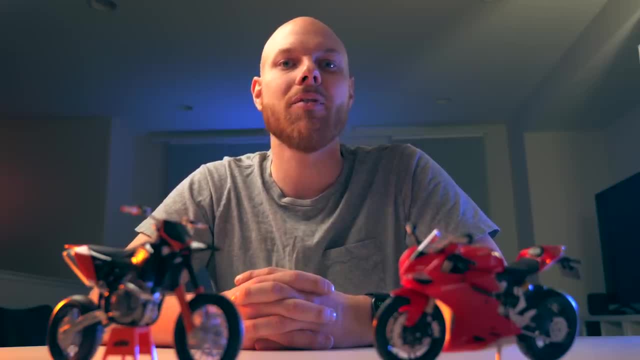 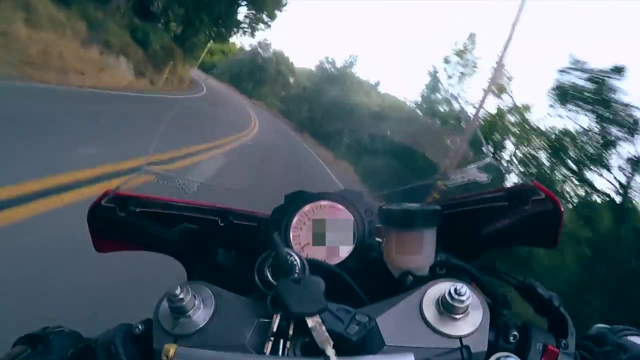 released is very important because it controls the amount of engine brake applied to the rear tire. Step 3. Turn in. The rider turns into the corner by counter steering or applying a quick torque to the handlebars in the opposite direction. Step 4. Turn in. The rider turns into the corner. 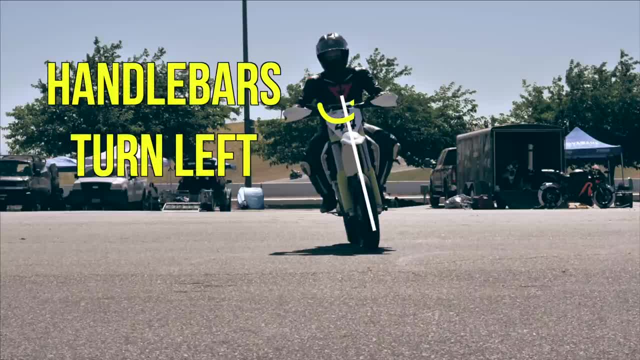 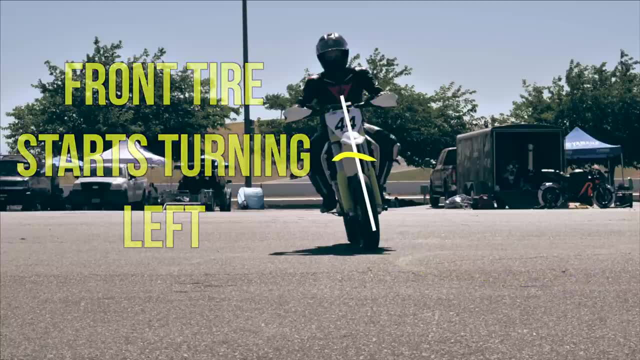 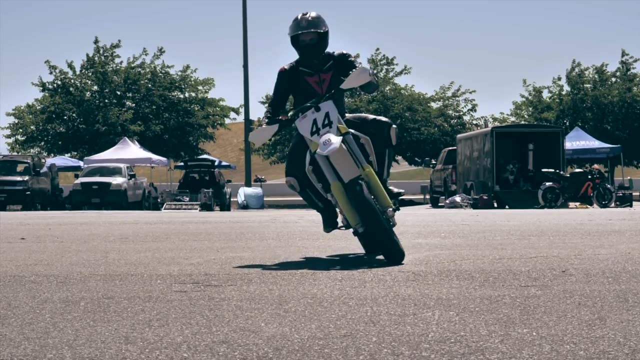 by counter steering or applying a quick torque to the handlebars. in the opposite direction, The movement of the front wheel around the steering head generates a front tire lateral force that has the effect of leaning the motorcycle into the turn. In addition to this, the gyroscopic effect generated by the front wheel and the steering 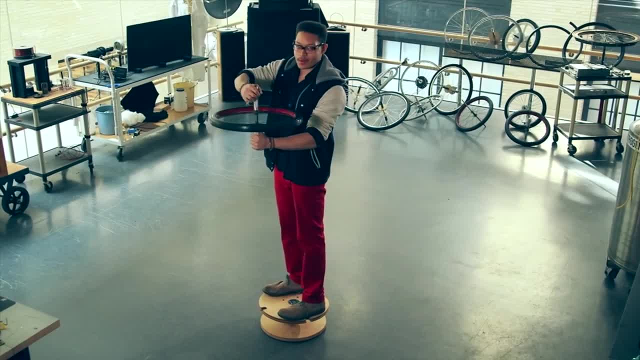 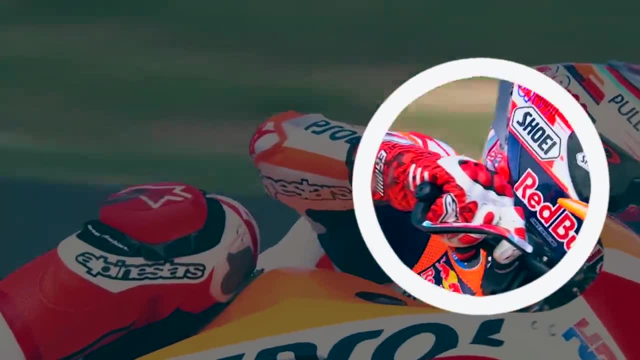 rotation causes a gyroscopic movement that also helps lean the bike into the turn, So the rider turns in. stay on the brakes using what is called trail braking, where the brakes are gradually released into the corner. You remember what is happening with the. 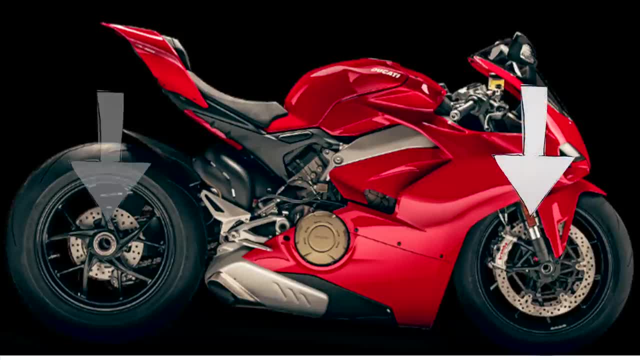 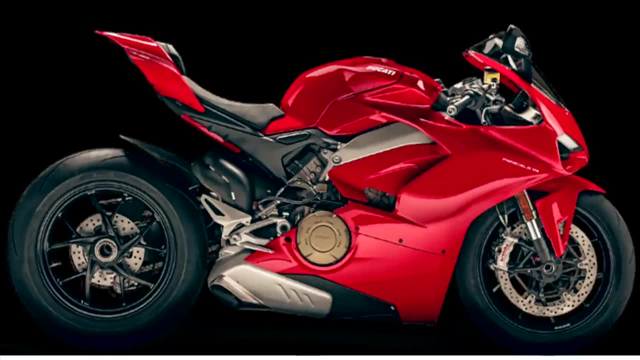 chassis. when the front brakes are applied, The front forks are compressed and the rear suspension is extended. What will happen if the front brakes are suddenly released? The front fork will extend, making it harder to steer in. since the trail is increased, It will transfer load to the rear tire. 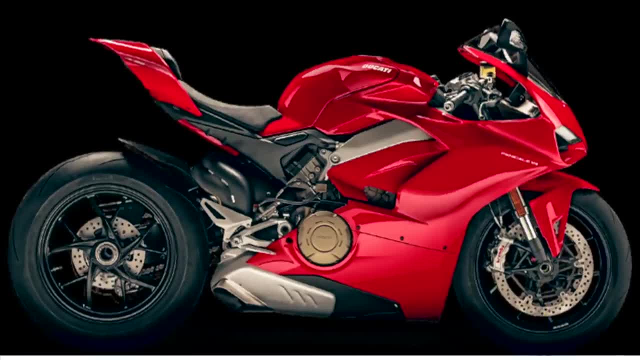 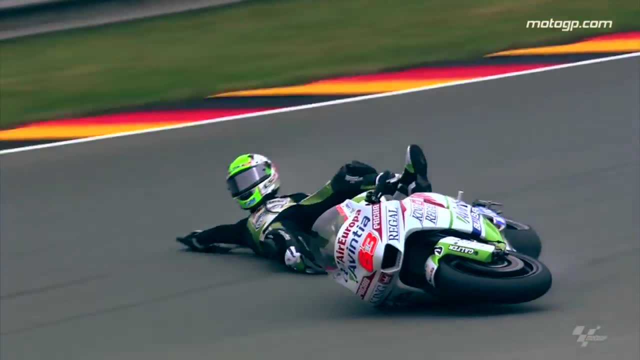 decreasing traction on the front. Step 5. Turn in. The rider turns in. stay on the brakes. furthermore, the movement of the front fork extending will destabilize the entire bike. If a rider does not trail brake, they will go into the corner like they're on a pogo stick. 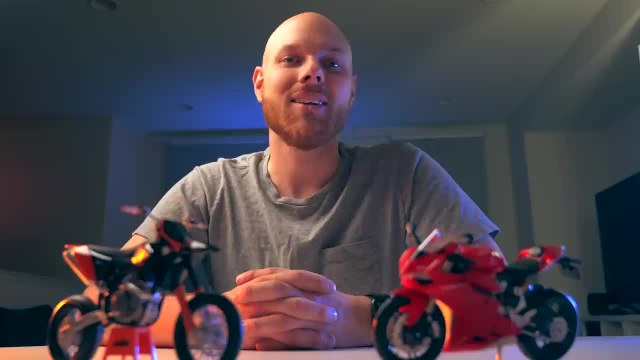 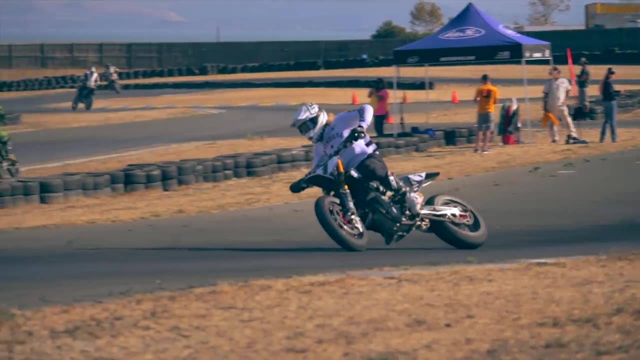 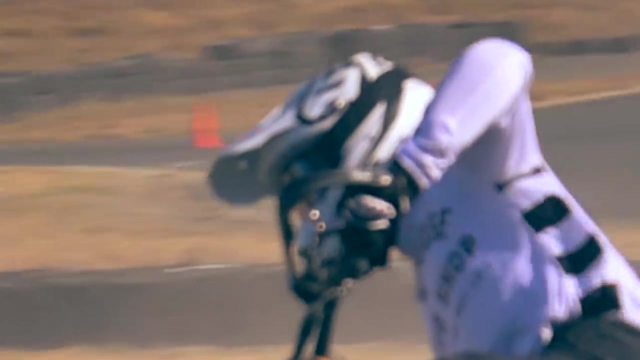 bouncing back and forth. Now, that is certainly not a desirable way to enter a corner at high speed. now is it So the rider is moving towards the apex. Remember I mentioned that when the clutch is released is very important. Step 6. Turn in. The rider turns in. stay on the brakes. 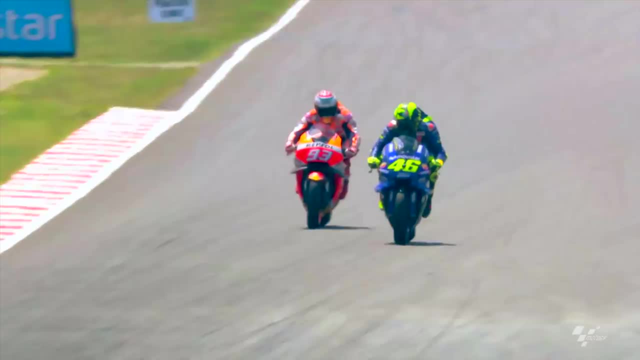 furthermore, the movement of the front fork extending will destabilize the entire bike. So the rider is moving towards the apex. Remember I mentioned that when the clutch is released is very important. Step 7. Turn in. The rider turns in. stay on the brakes. furthermore, the movement of the front fork extending will destabilize the entire bike. 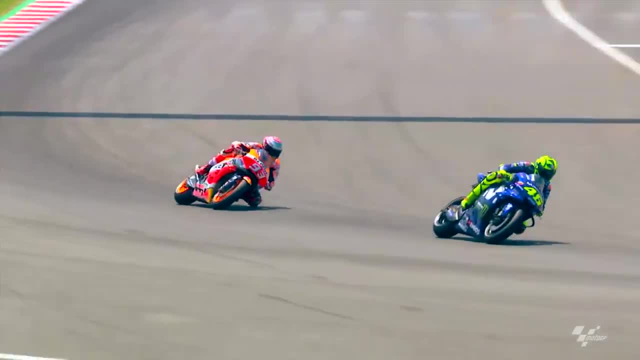 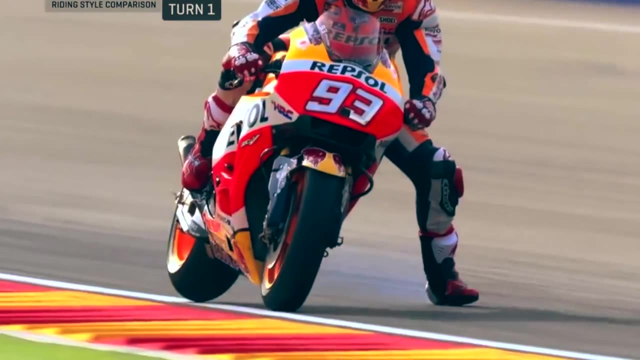 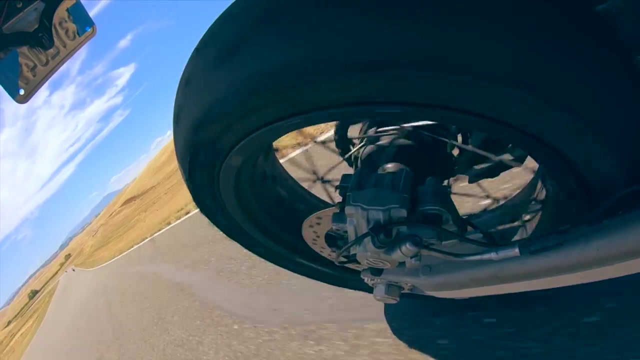 You've probably seen riders backing it in where the rear wheel comes out into a slide. The slide is caused by two major things: 1. The weight transfers forward caused by applying the front brake and the rider moving forward, which makes the rear wheel light. 2. The rear wheel being slowed down by engine braking. 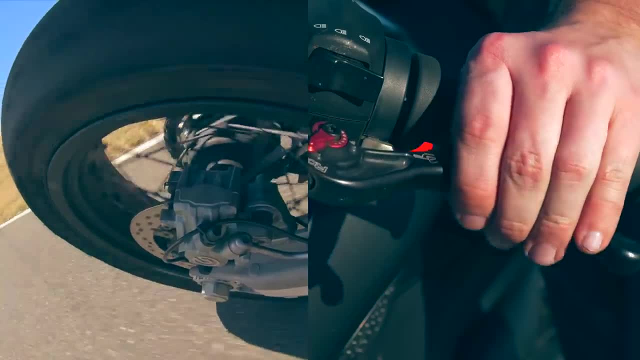 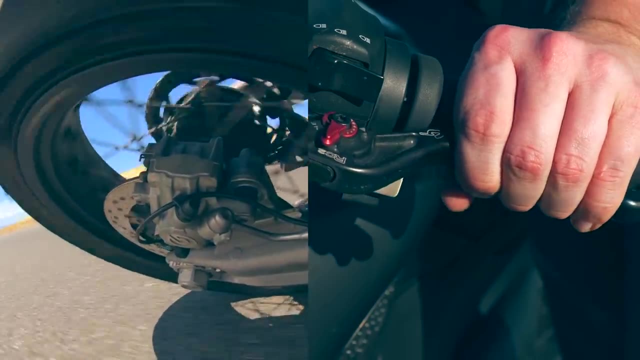 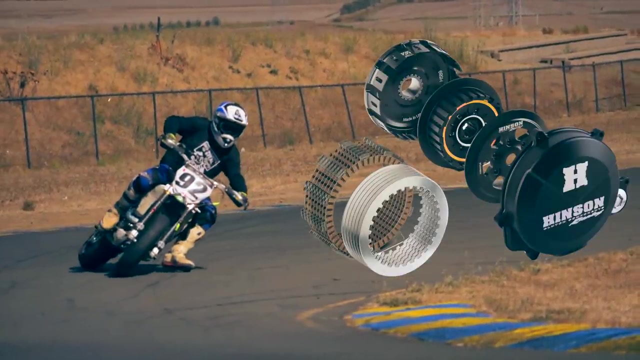 application of rear brake or both at the same time. Engine braking can be controlled by modulating the clutch, So in other words, the rider can control how much the rear wheel slips by working the clutch. Now, pretty much all modern race bikes come standard with something called a 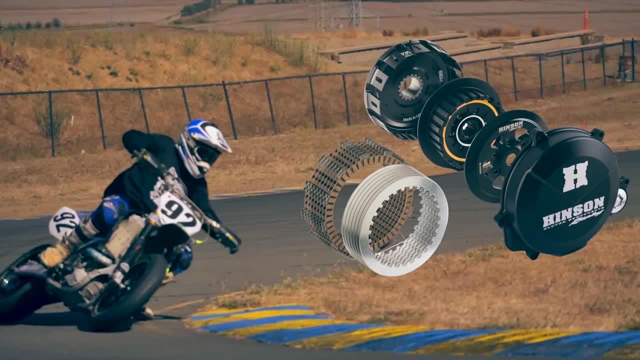 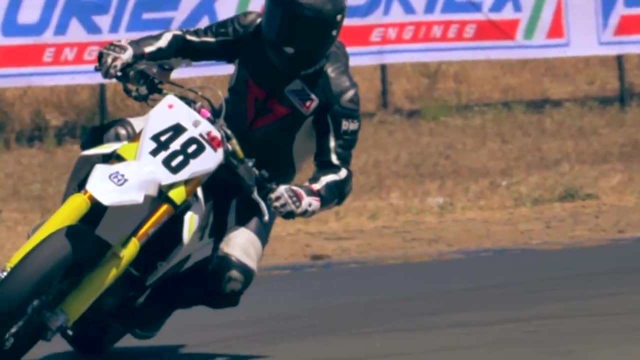 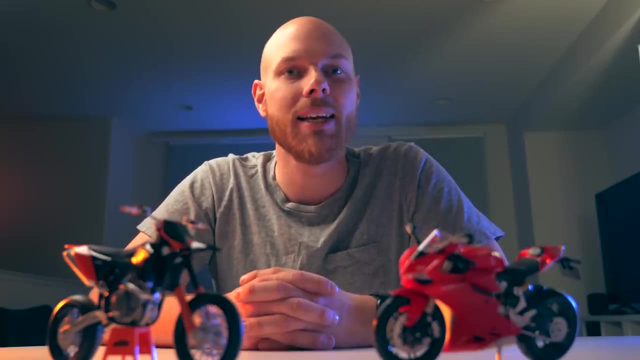 slipper clutch, which enables the rider to release the clutch quite rapidly without getting the rear wheel hop. So some riders will release the clutch completely before entering the corner. Sometimes they don't completely release the clutch. and now we get to answering one of the questions posed in the beginning of the video. 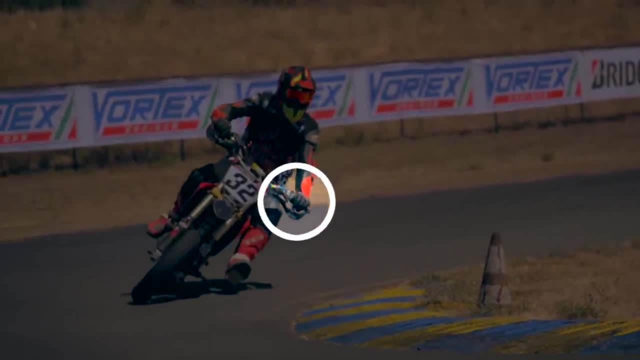 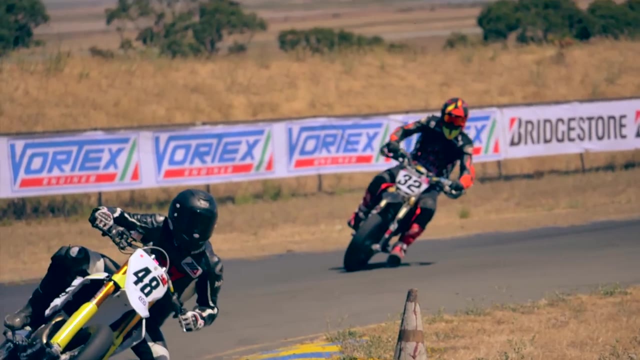 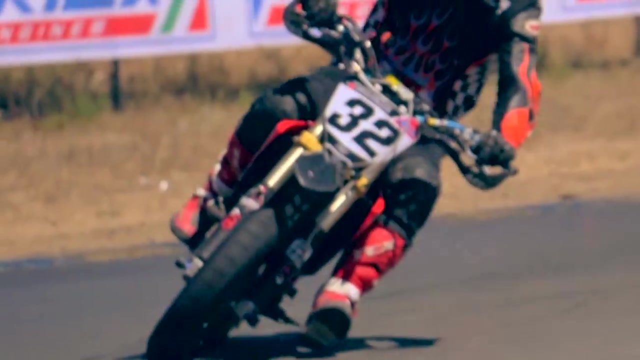 video: Why is Piers pulling the clutch all the way into the corner? You already know the answer to the question, don't you? He is controlling the rear end slide by modulating the clutch and working the rear brake. In fact, we can even see that he is releasing the rear brake at exactly the same time as 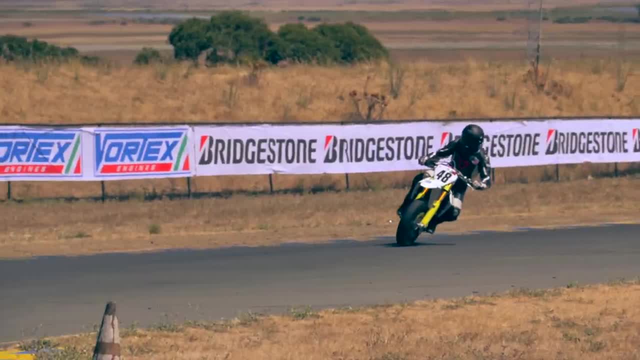 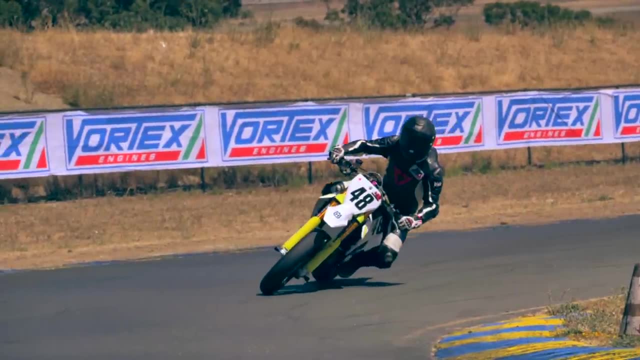 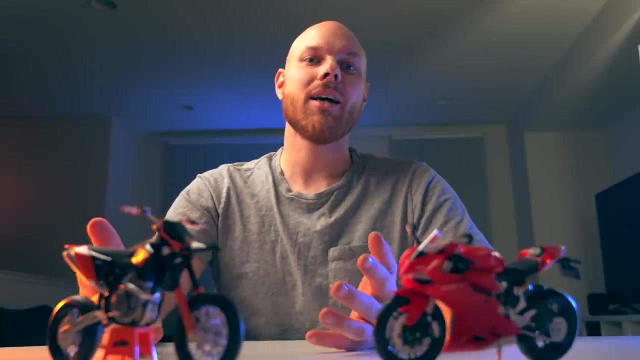 he is releasing the clutch. Here is a racer going through the same corner by using both engine brake and rear brake, completely releasing the clutch before the corner. So why would you choose one over the other? Well, it simply comes down to personal preference of the rider. 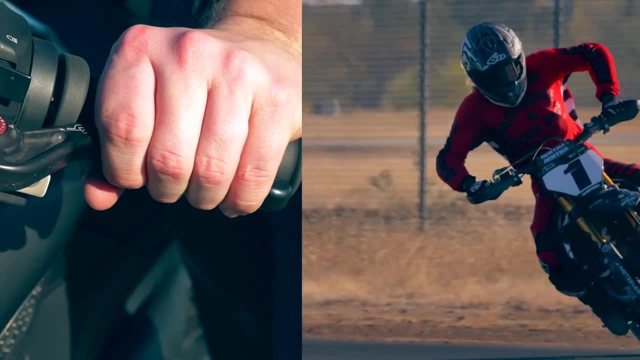 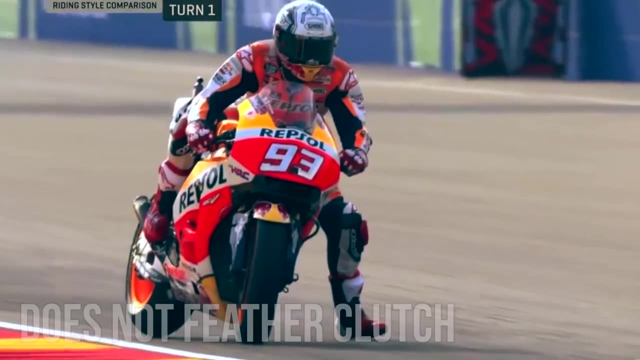 Using the clutch gives more direct control over the slide as compared to just releasing the clutch. This is because if you pull in the clutch and release the rear brake, the slide will stop. So a rider who is already pulling on the clutch can regain traction much faster than a rider. 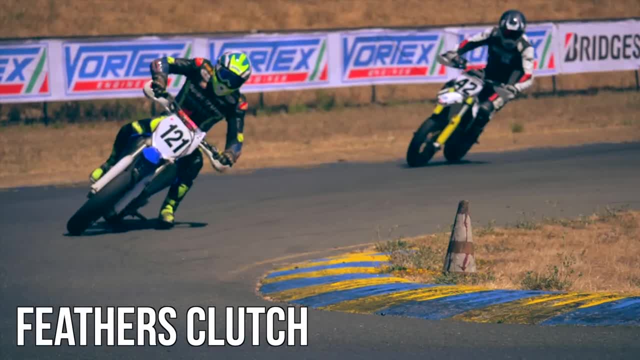 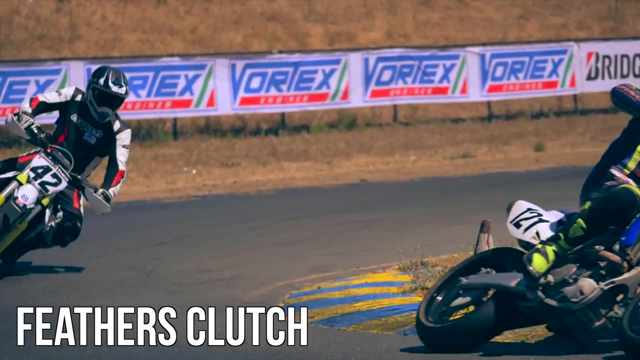 who has to reach the clutch. The downside of using the clutch and rear brake is, of course, that it requires a lot from the rider to control all of that at the same time. If the rider uses a superbike riding style, they will move their upper body with the bike. 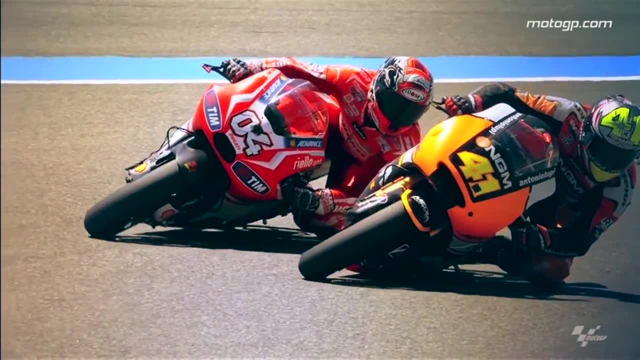 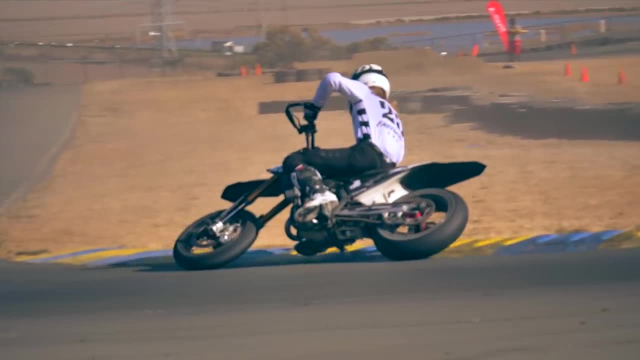 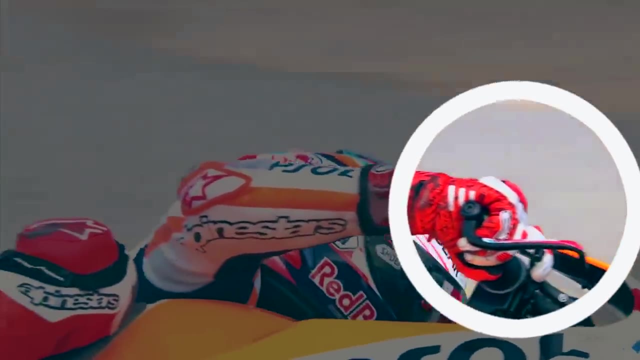 as it leans into the corner, basically diving inside Step 4.. Mid-corner: The rider is moving towards the apex of the corner, gradually releasing the front brake. As soon as the front brake is released, the rider starts twisting. So why does Marquez flick his hand after releasing the brakes? 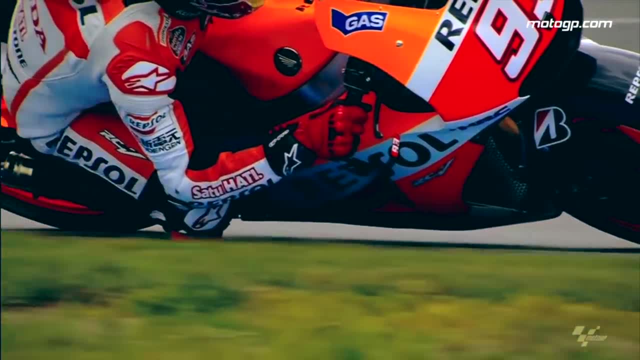 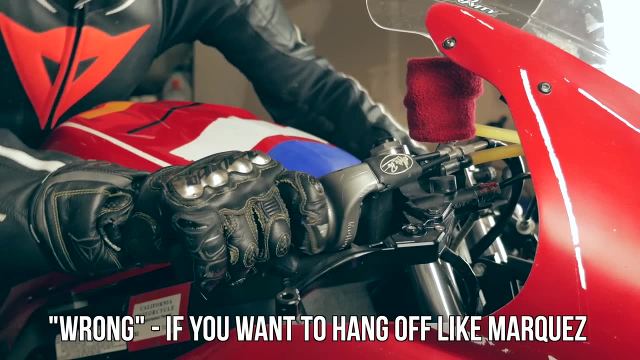 Well, it's for two reasons. One, to be able to accurately control the throttle input. Two, to be able to move his right elbow freely. You see, if he doesn't shift his grip around the handlebars, he would lock his elbow in. 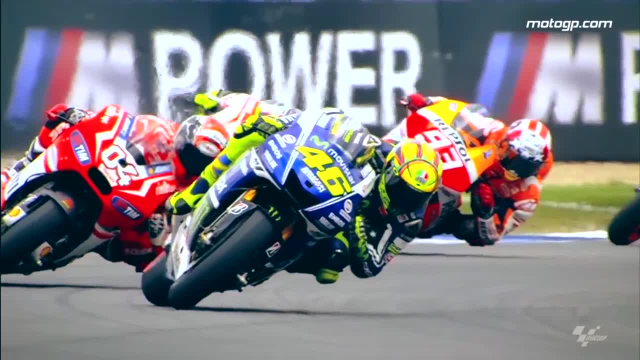 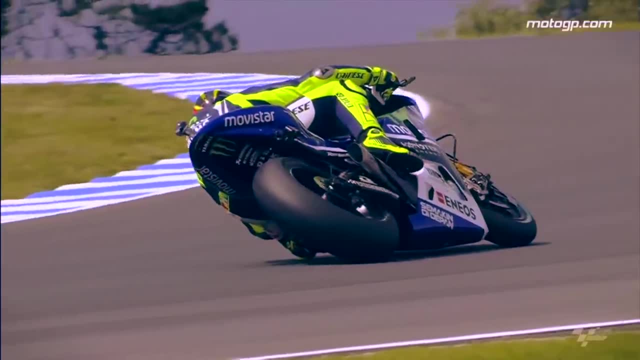 a way that does not allow him to move freely. If turning left, he will extend his arm over the tank. If turning right, he pushes his elbow into the turn. This leads nicely into the question: why is Rossi pushing his upper body down even more? 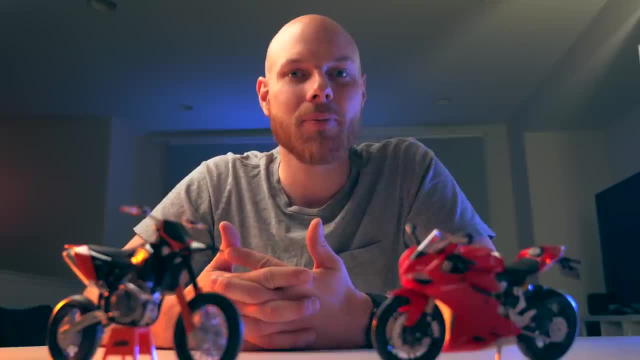 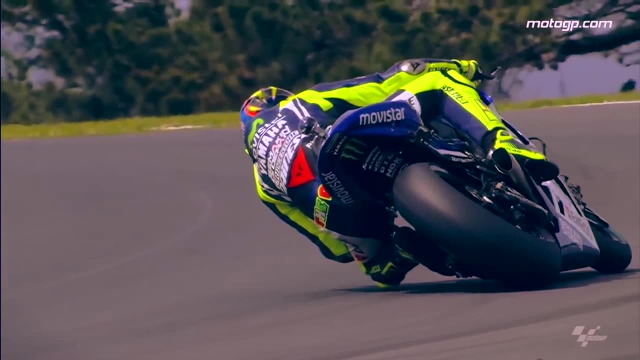 in the middle of the corner. So why is he doing this? Well, it's quite simple: He's tightening up his line so that he can be on the throttle harder and accelerate out from the corner faster. You see, when a rider hangs off to the inside of the motorcycle, this transfers the combined 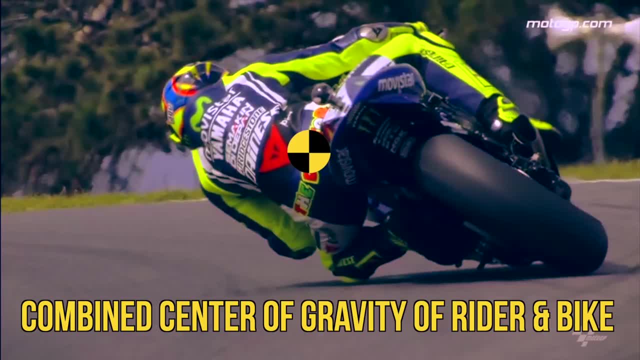 center of gravity of them and the bike, which enables less lean angle, at the same speed. If the lean angle is kept constant but the rider is not able to keep up with the speed, the rider will be able to keep up with the speed. 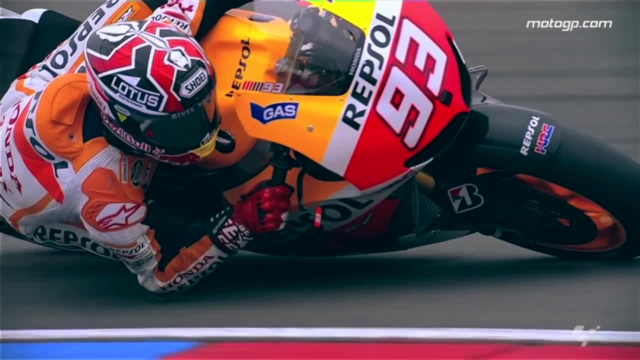 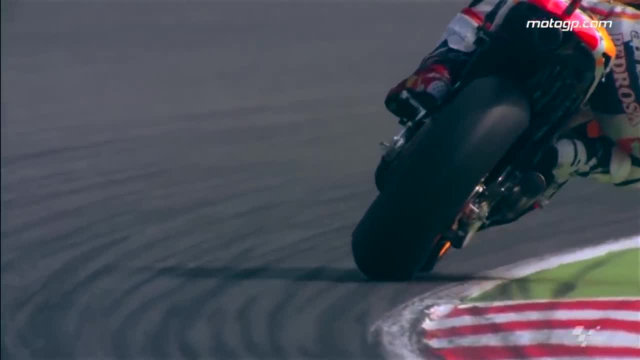 If the rider moves their upper body even further into the corner, they will tighten up their line. If they are on the throttle, it will enable them to keep the bike as upright as possible during this crucial part of the corner. So, ladies and gentlemen, I know you've been waiting for this one. 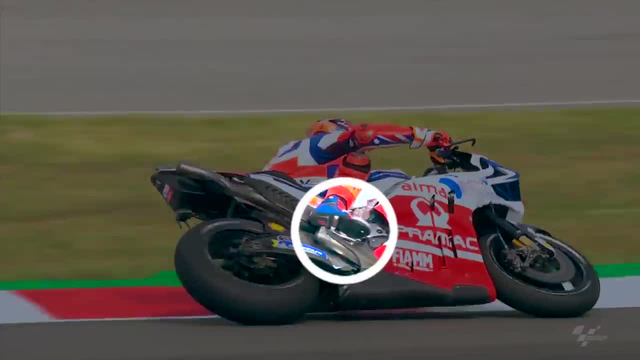 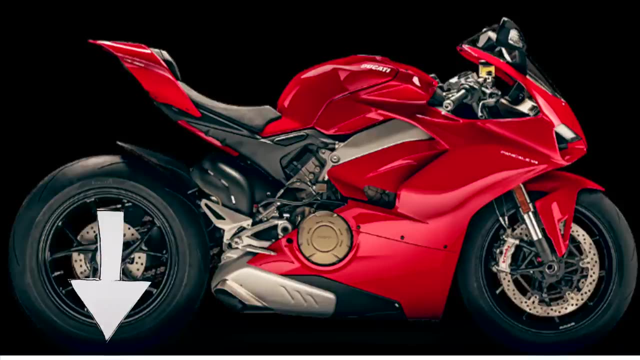 Why is Miller applying the rear brake in the middle of the corner? Let's again have a look at the chassis geometry. at this point in the corner, The rider is releasing the front brake. This will transfer load to the rear, which is good, since the rider is soon going to be. 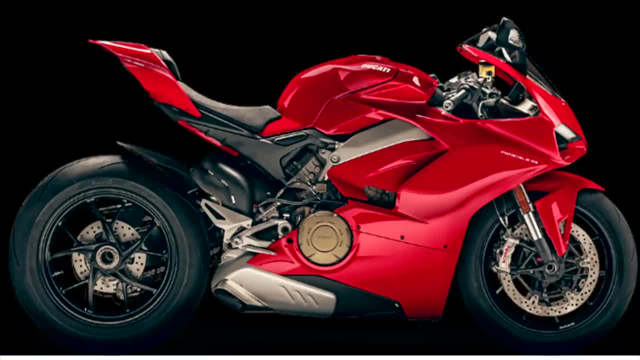 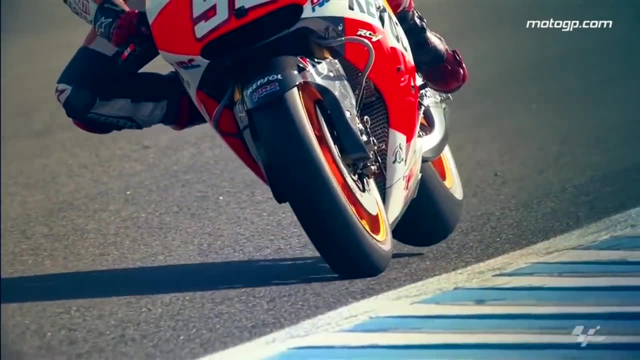 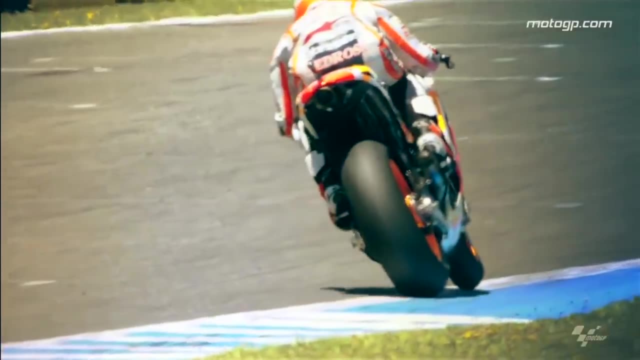 applying throttle, which will require traction from the rear tire. This will also increase the trail, further stabilizing the bike, Though we should also remember that when the front brakes were being applied, the rear suspension was extended, which decreased the wheelbase, and the rear suspension is potentially 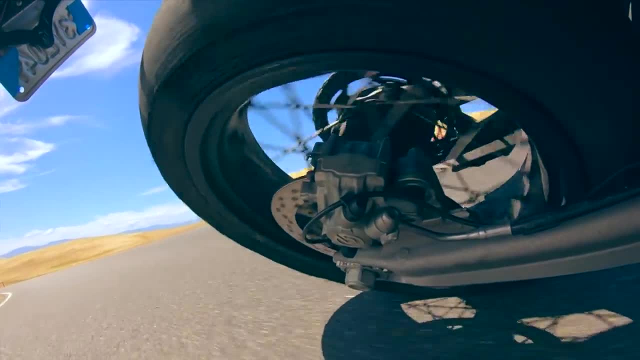 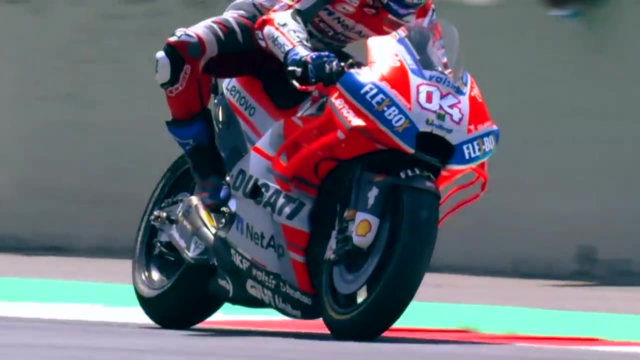 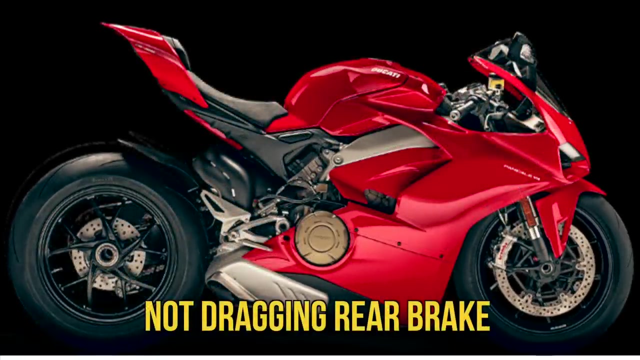 so extended that it won't follow down bumps as efficiently. It is outside of its optimum range. What can an expert rider do about this? What can an expert rider do about this? Drag the rear brake. By dragging the rear brake, the rear suspension is kept in check and the wheelbase is extended. 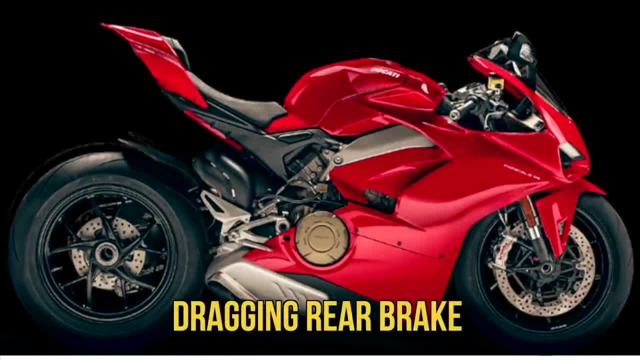 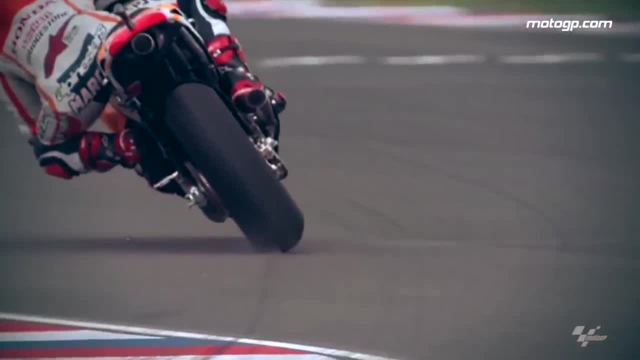 which stabilizes the bike. They are dragging the brake enough to cause this geometry change, but not so much that they are slowing down to any large extent. They now have a chassis geometry that works well to get on the throttle and drive them out of the corner. 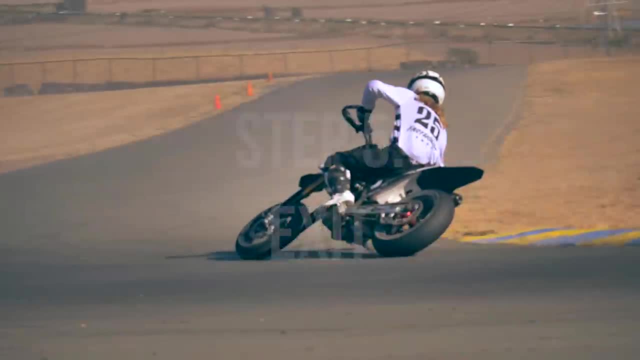 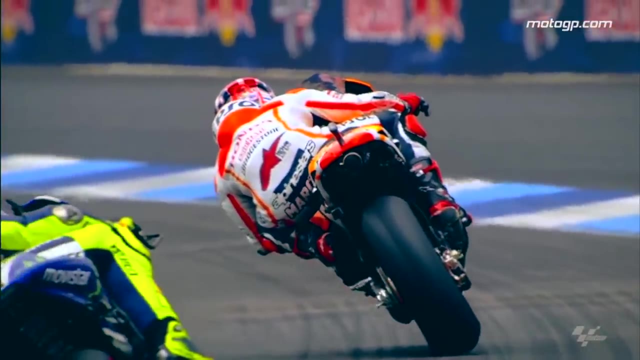 Kinda cool, huh. Step 5. Exit: The rider is smoothly adding more throttle, throttle going out of the corner In their superbike riding style. in order to get as much traction out of the corner as possible, the rider stays to the inside of the bike and does not follow the bike up. 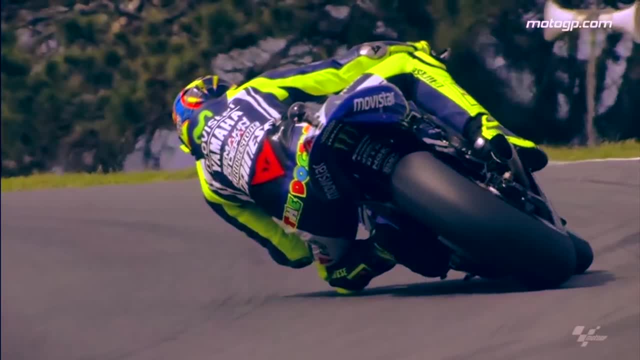 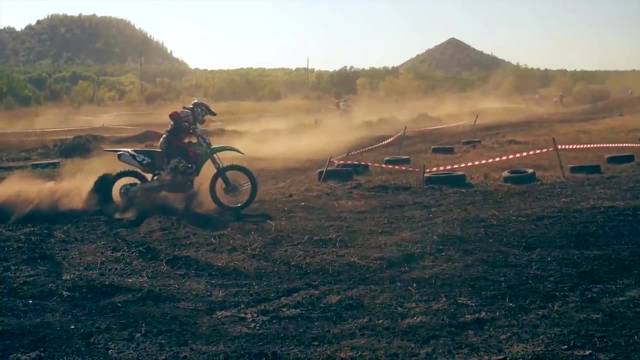 This is simply to have as small amount of lean as possible, enabling greater acceleration. In a pure dirt bike riding style, the rider would stay on top of the bike and straight and out with the bike. In the dirt, the bike is going to be sliding around, since there isn't much traction. 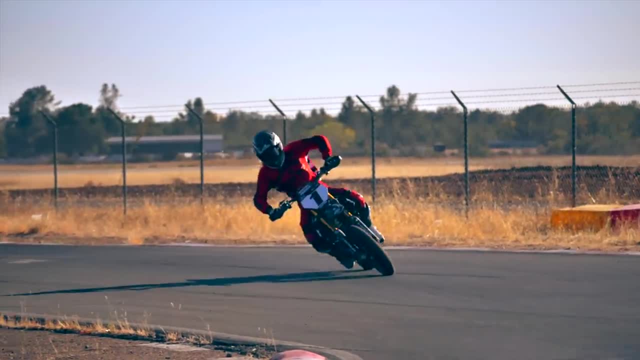 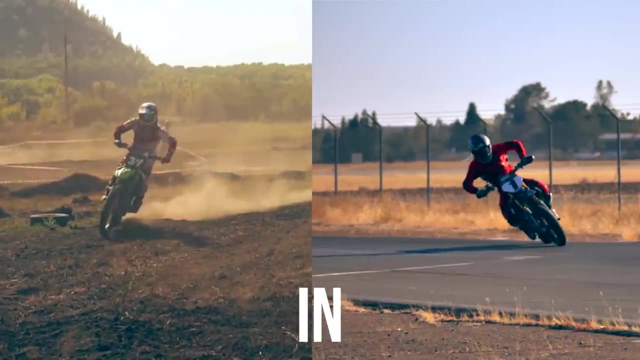 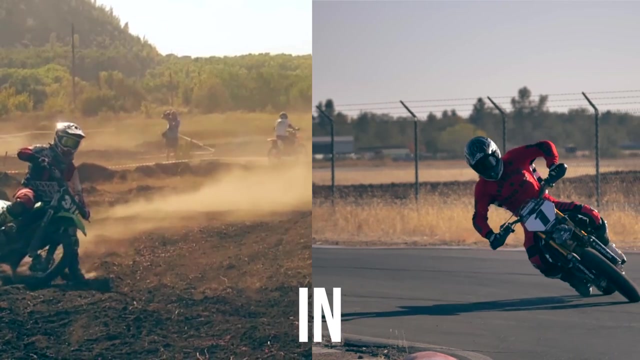 So why is McAllister pushing the bike down, going into the corner, but then leaning his upper body into the corner on the exit? He is combining dirt bike and superbike riding styles to go through the corner as quickly as possible. He is pushing the bike down, going into the corner in order to control the rear end slide. 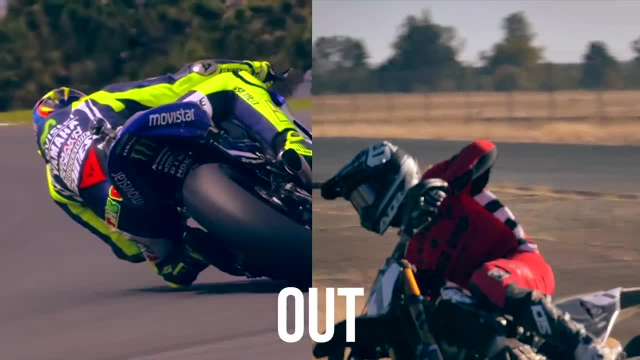 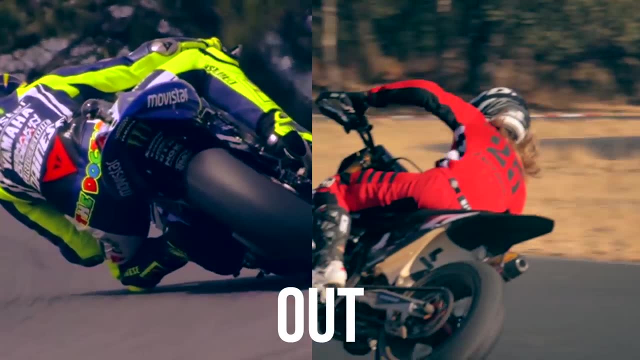 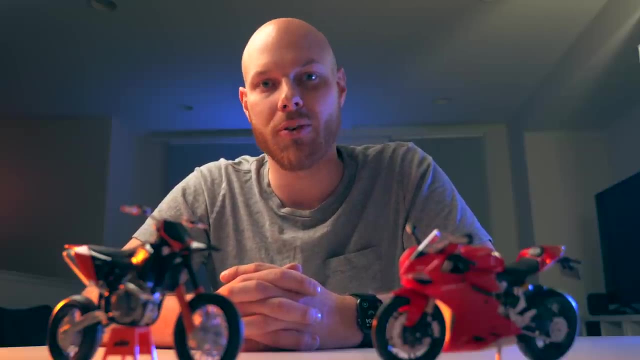 but on the exit he wants as little lean angle as possible to maximize the drive out of the corner, So he leans to the inside. I hope you've learned something today and that this has sparked an interest in you for motorcycle dynamics as well as cornering technique. 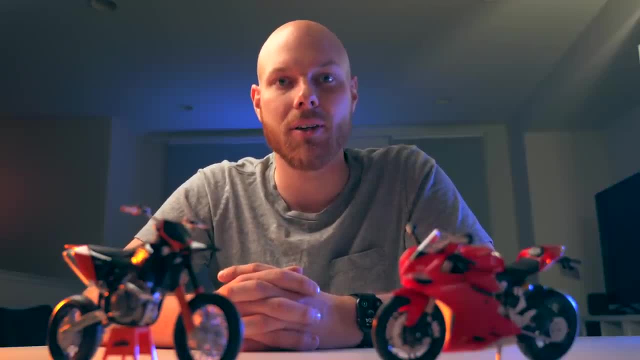 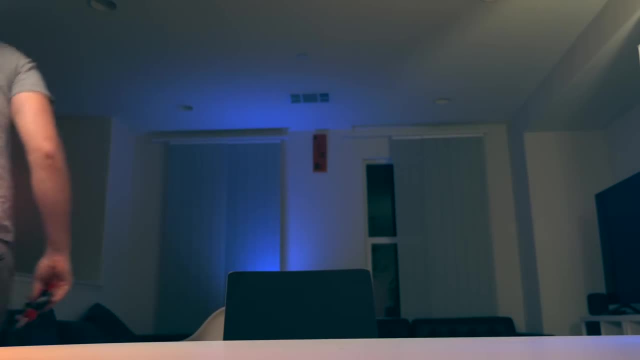 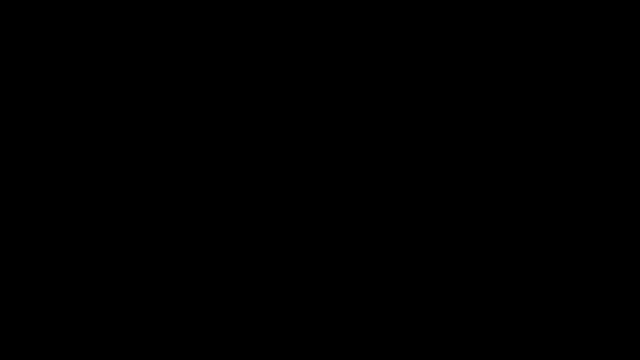 Feel free to question any of my assertions down in the comment section. That's it for today. over and out, Have a great day.